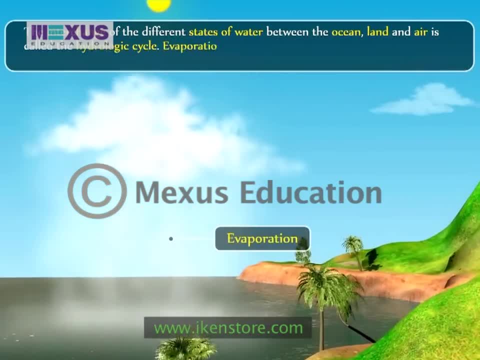 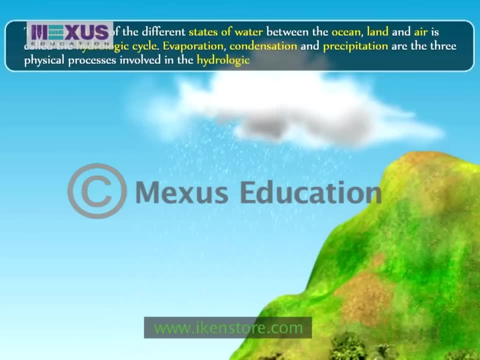 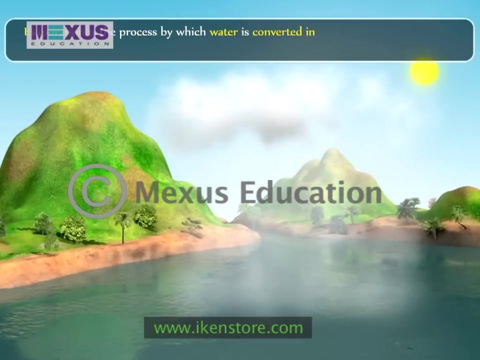 is called the hydrologic cycle. Evaporation, condensation and precipitation are the three physical processes involved in the hydrologic cycle. Evaporation is the process by which water is converted into water vapor by the sun's heat. The rate of evaporation is directly. 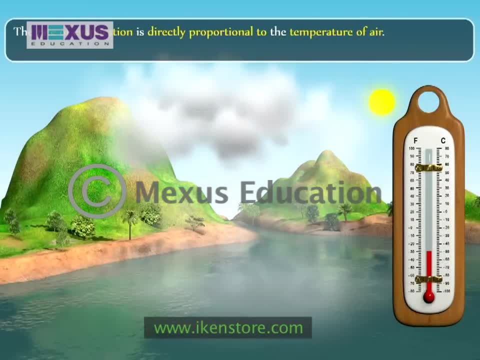 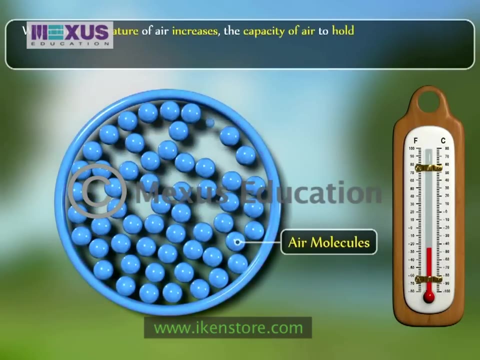 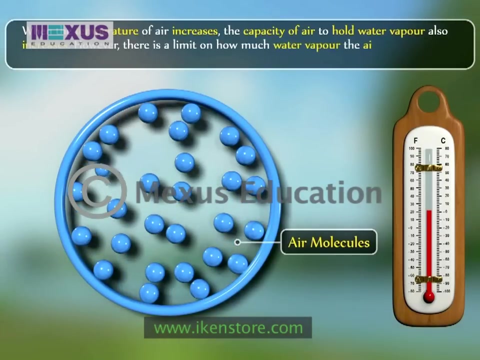 proportional to the temperature of air. Evaporation occurs at all temperatures. However, it is more rapid at higher temperatures as compared to lower temperatures. When the temperature of air increases, the capacity of air to hold water vapor also increases. However, there is a limit on how much water vapor the air can hold at any given temperature. 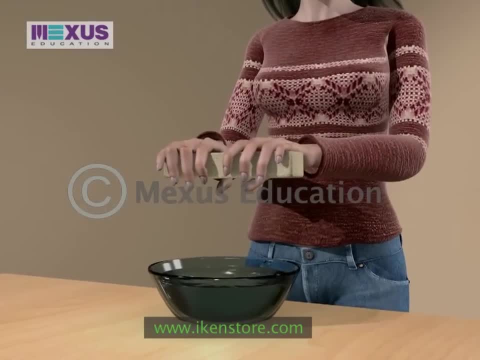 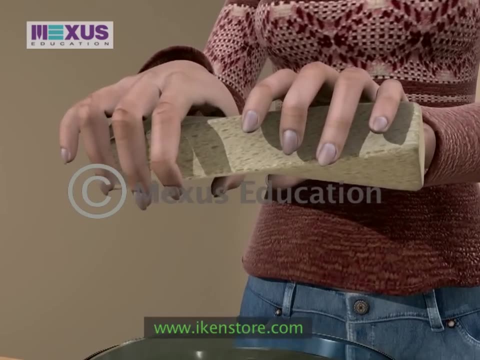 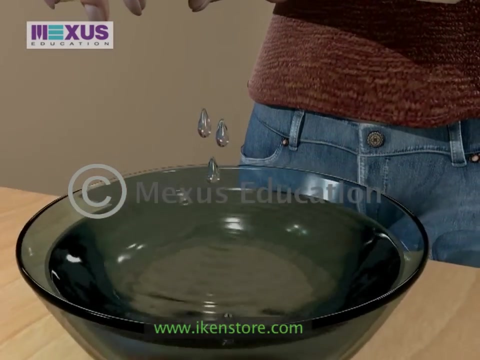 A mass of air is like a sponge. Lowering the temperature of a mass of air is like squeezing a sponge. If you squeeze a soaking wet sponge, water will drip out of it, since the capacity of the sponge to hold water decreases. But damp sponge requires a good squeeze to wring all the. 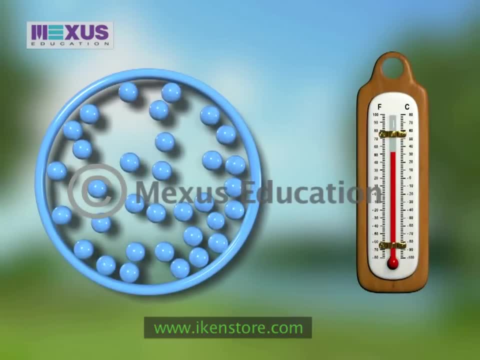 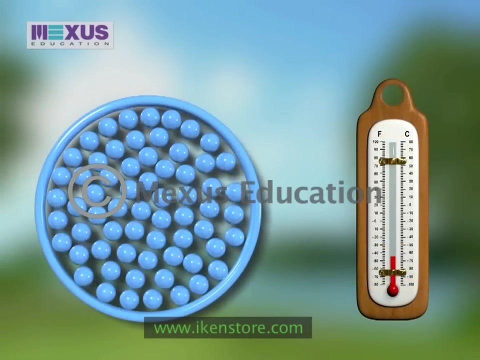 water from it. Similarly, when the temperature of air decreases, the capacity of the air to hold water vapor decreases, and when the temperature increases, the capacity of the air to hold water vapor increases When the air is holding the maximum amount of water. 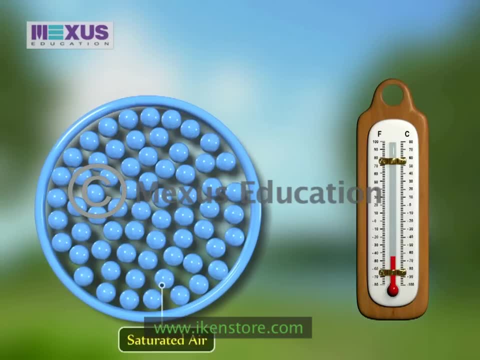 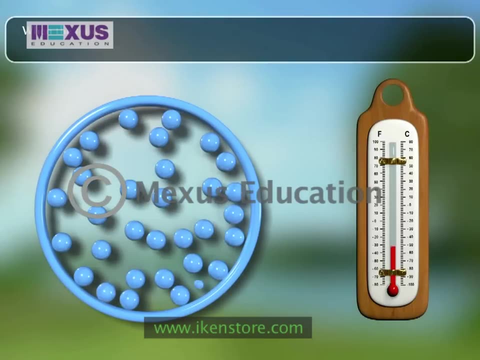 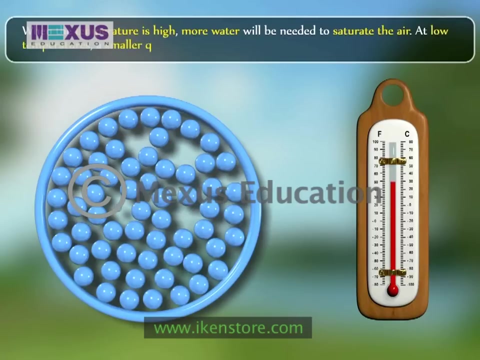 it can hold the air is said to be saturated. The capacity of air to hold water is related to the temperature. When the temperature is high, more water will be needed to saturate the air. At low temperatures, a smaller quantity of water would be enough to saturate the air. The temperature: 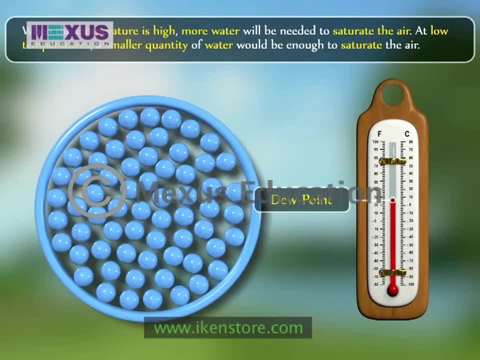 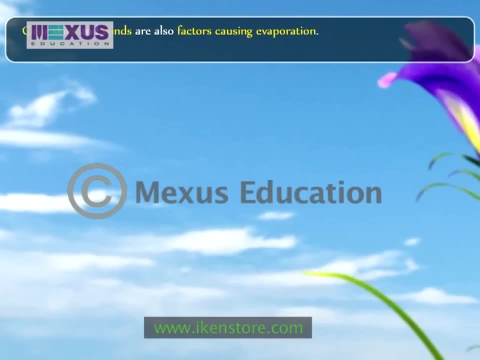 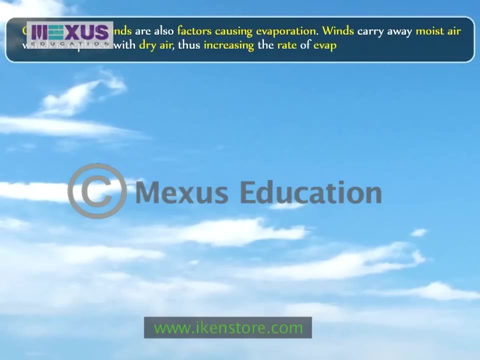 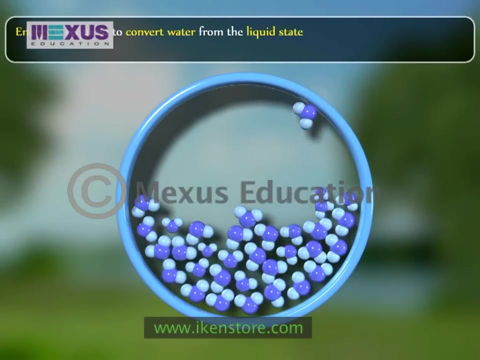 at which the air gets saturated is known as the dew point. Clear skies and winds are also factors causing evaporation. Winds carry away moist air, which is replaced with dry air, thus increasing the risk of evaporation rate of evaporation. Energy is required to convert water from the liquid state to the 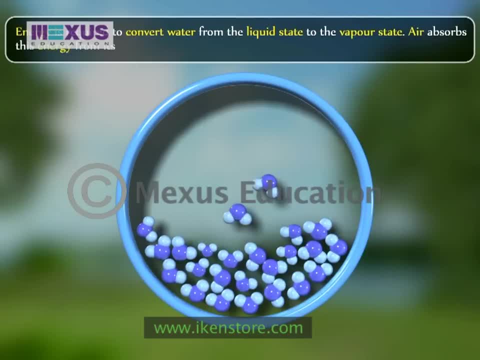 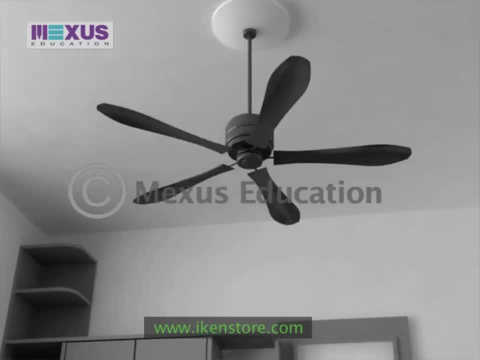 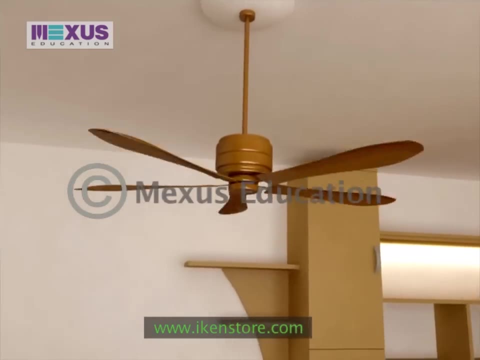 vapor state Air absorbs this energy from its immediate surroundings. For example, on a hot day, it feels cool under the fan because the perspiration of the skin evaporates quickly due to the rapidly moving air. As the moisture evaporates, it absorbs heat from the skin. 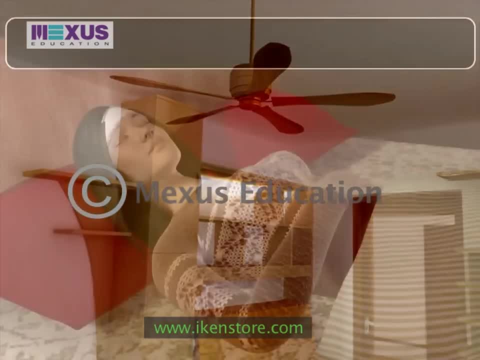 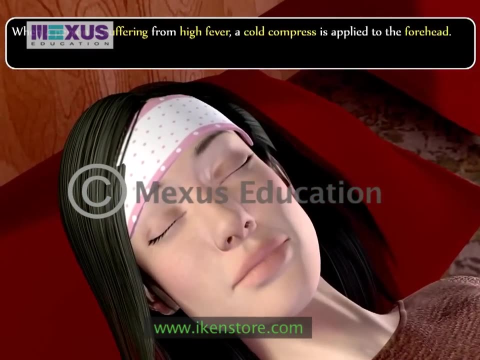 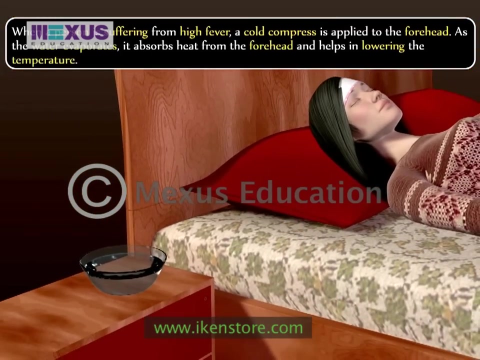 surface, causing it to cool. When a person is suffering from high fever, a cold compress is applied to the forehead. As the water evaporates, it absorbs heat from the forehead and helps in lowering the temperature. The term humidity refers to the amount of water vapor present. 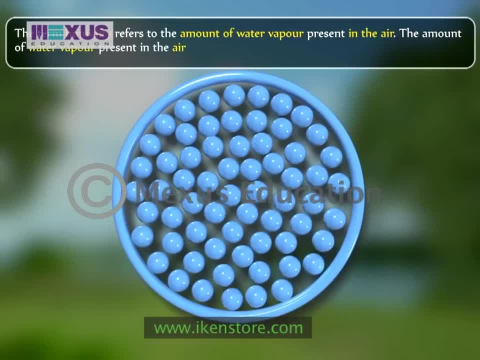 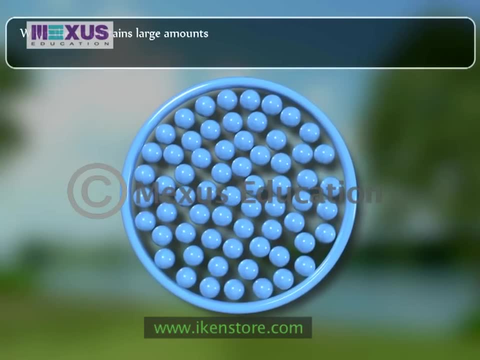 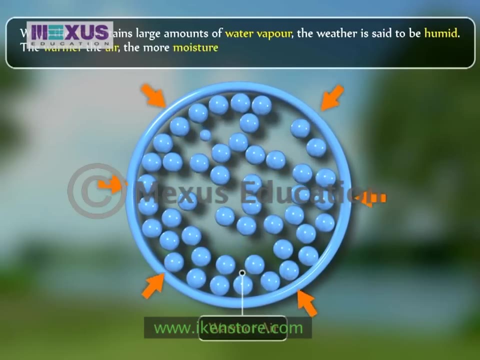 in the air. The amount of water vapor present in the air varies greatly from time to time, and from time to time When the air contains large amounts of water vapor, the weather is said to be humid. The warmer the air, the more moisture it can hold. The total amount of water vapor present in 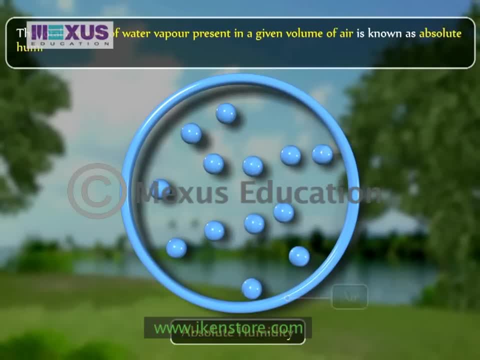 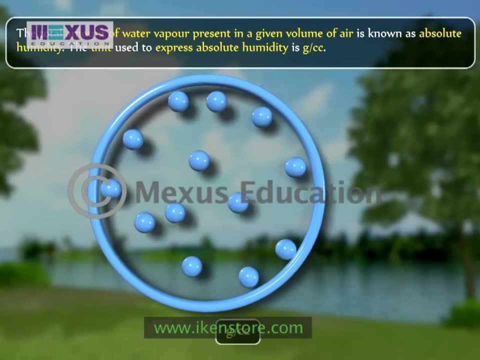 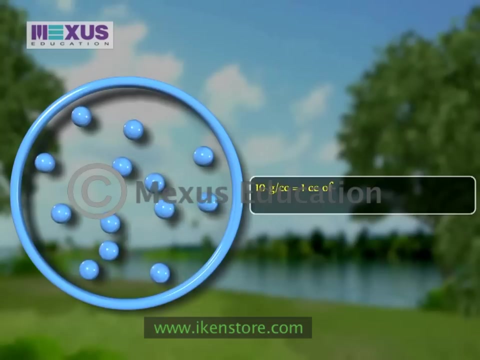 a given volume of air is known as absolute humidity. The unit used to express absolute humidity is grams per cubic centimeter. If the absolute humidity is expressed in a given volume of air, it equals a little more than an actual fluid. The reason for this is because low humidity is not normal. If water vapor is expressed in absolute humidity has meaning after other total noises. it means that the humidity is expressed If even one wire isested in an infinite amount. the humidity is expected to decrease as time passes. 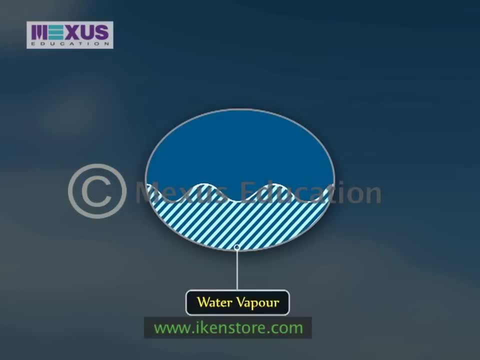 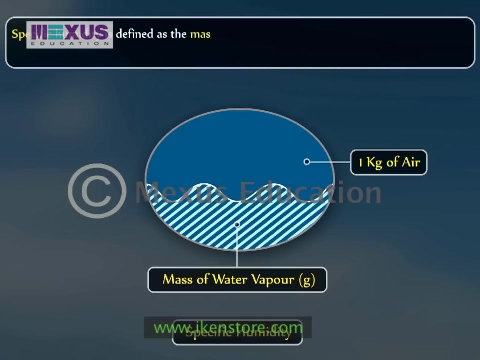 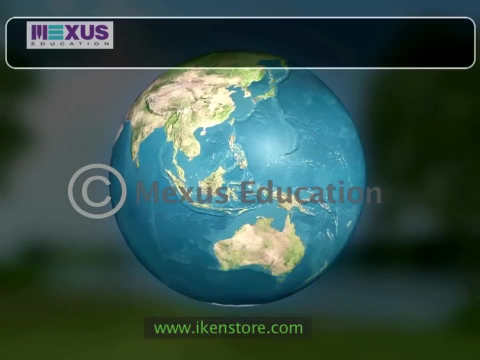 If oil is leaving the air, it indicates that it has reached the actual water vapor present in a given volume of air. there is a maximum mass of water vapor that a kilogram of air can hold. specific humidity, therefore, is defined as the mass of water vapor in grams contained in one kilogram of air specific. 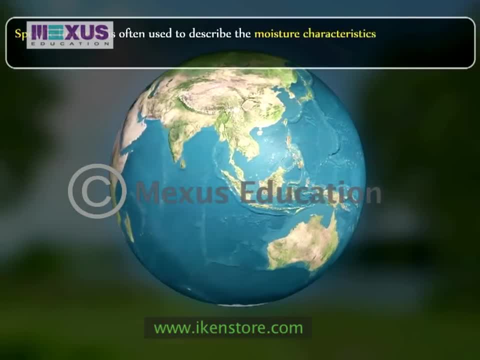 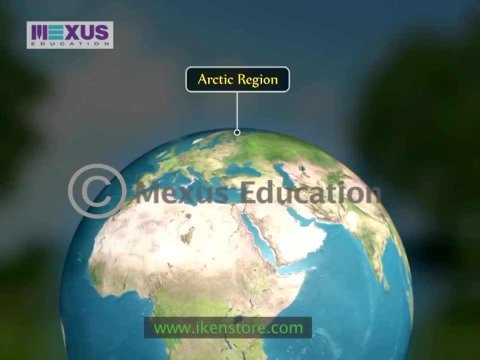 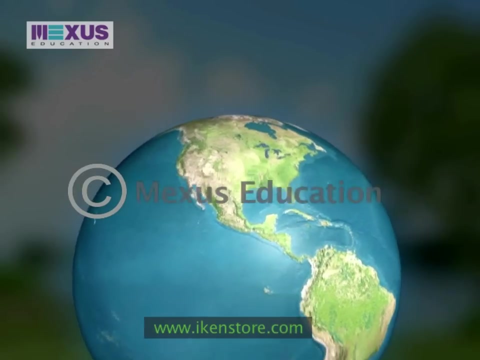 humidity is often used to describe the moisture characteristics of a large mass of air. for example, extremely cold, dry air over the Arctic region in winter may have a specific humidity as 0.2 gram per kilogram, while extremely warm, moist air of equatorial regions may have a. 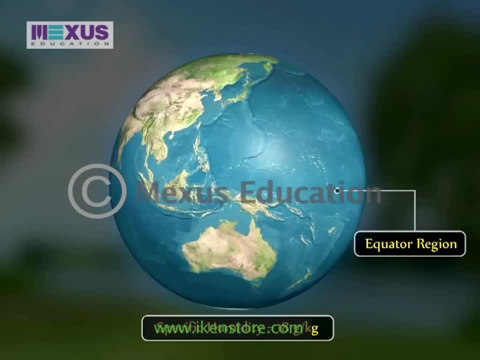 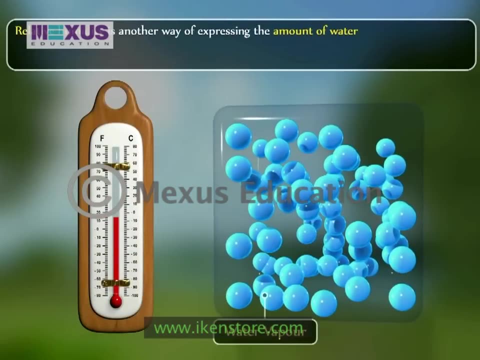 specific humidity as high as 18 gram per kilogram. relative humidity is another way of expressing the amount of water vapor in the air. it is a ratio between the actual amount of water vapor present in the in the area of atomization and coastal garbage�. Walter Jensen has given an explanation to. 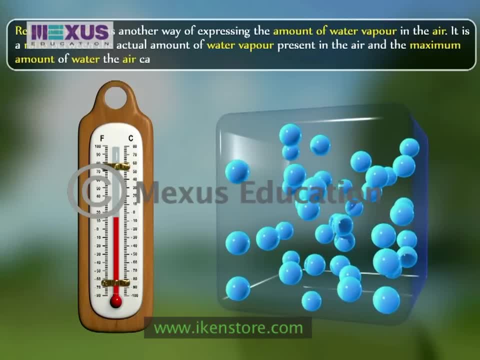 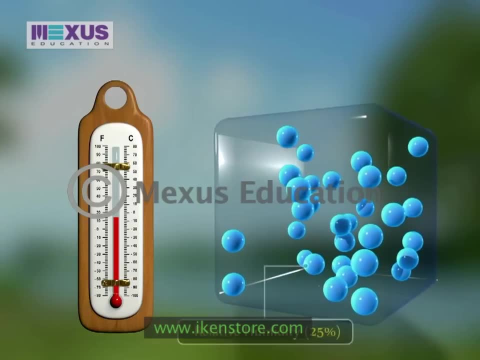 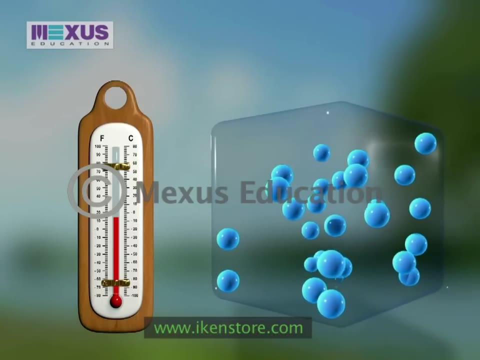 the air and the maximum amount of water the air can hold at that temperature. It is always expressed in percentage. For example, if the relative humidity is 25%, then it means that the humidity is not very high. It is only a quarter of its total capacity to hold water. 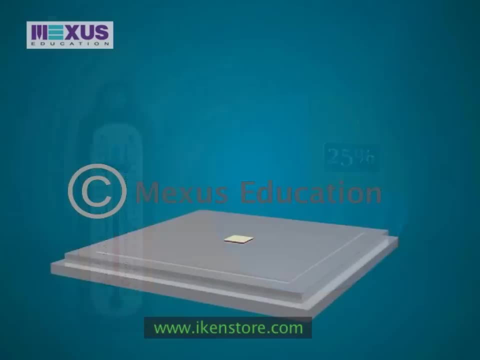 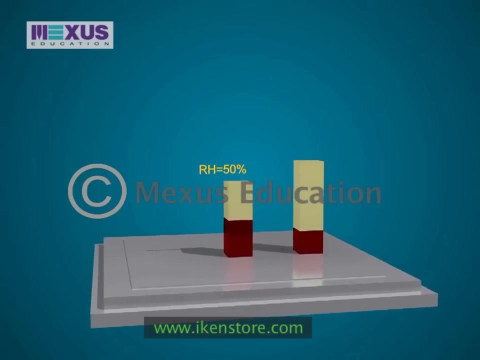 vapor at that temperature. Consider this graph: At 10 am, air temperature is 16 degrees Celsius and the relative humidity is 50%. By 3 pm, the air is warmed to 32 degrees Celsius by the sun and the relative humidity automatically drops to 25%, which is very dry air. The air becomes 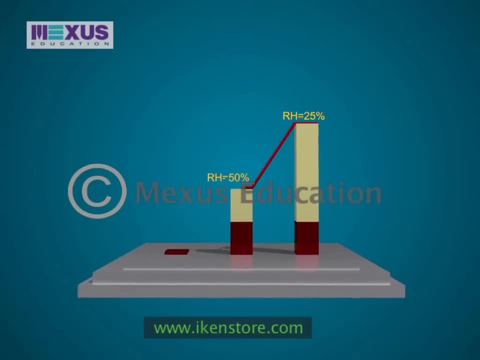 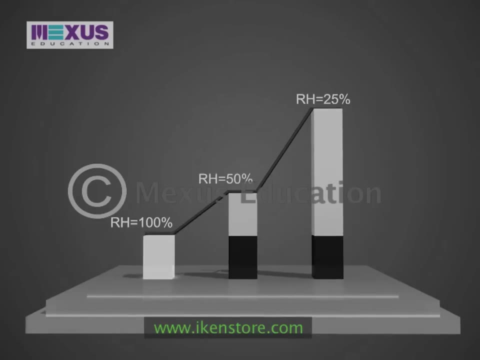 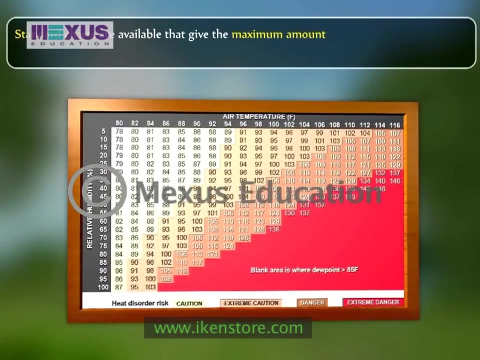 chilled during the night and by 4 am the temperature drops to 5 degrees Celsius. Now the relative humidity is automatically risen to 100% and the air is saturated. Standard charts are available that give the maximum amount of water the air can hold at different 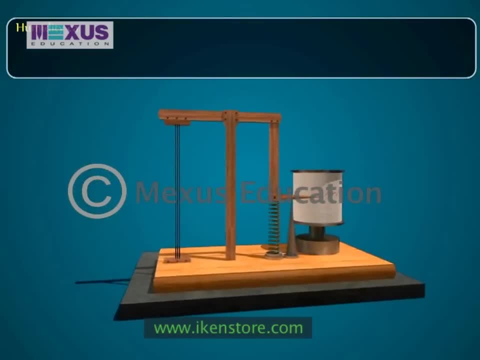 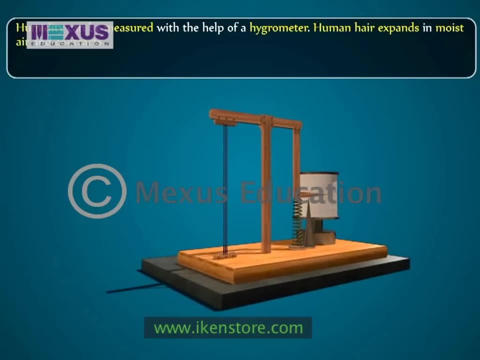 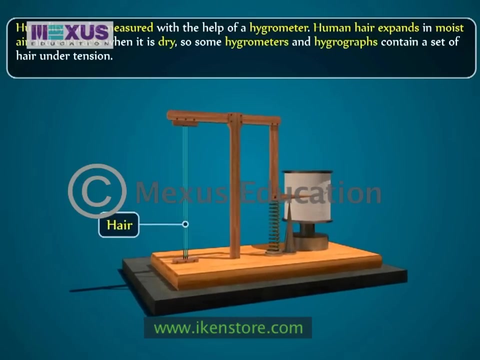 temperatures, Humidity, can be measured with the help of a hygrometer. Human hair expands in moist air and contracts when it is dry, So some hygrometers and hygrographs contain a set of hair under tension. Variation in the length of the hair: 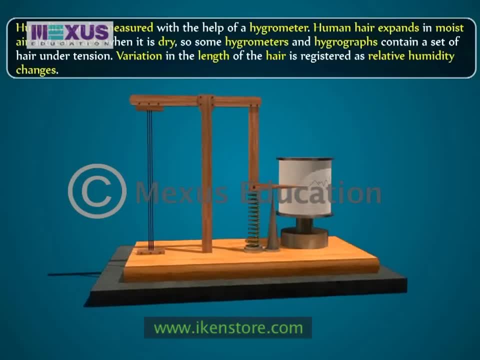 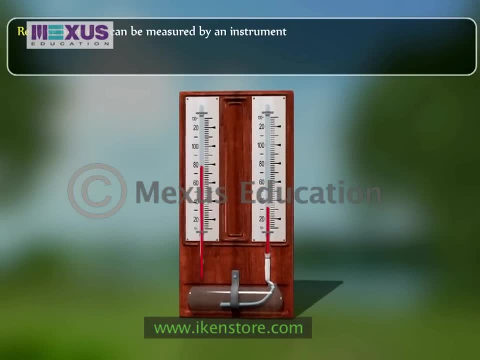 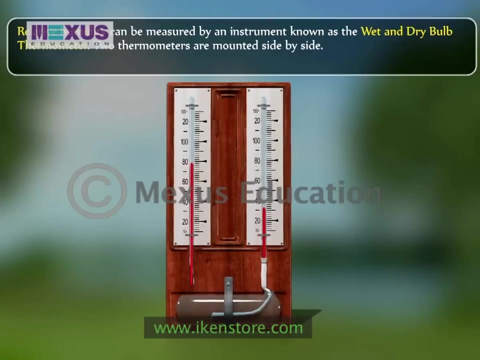 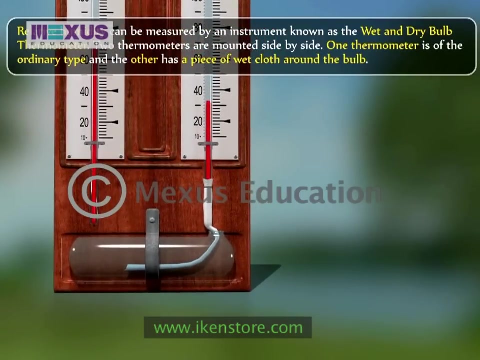 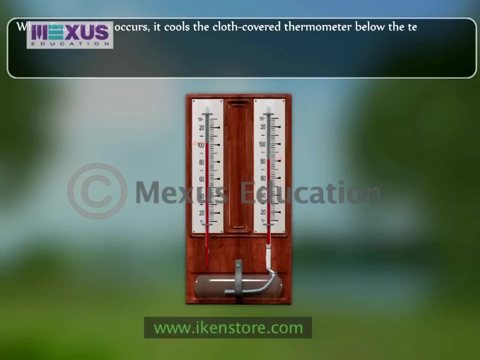 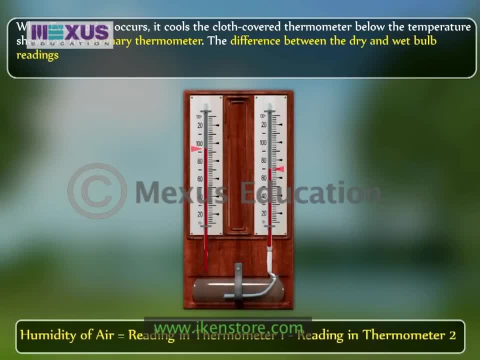 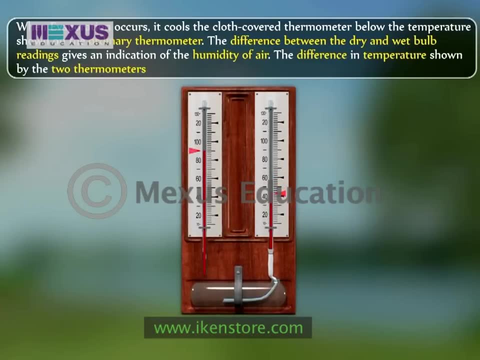 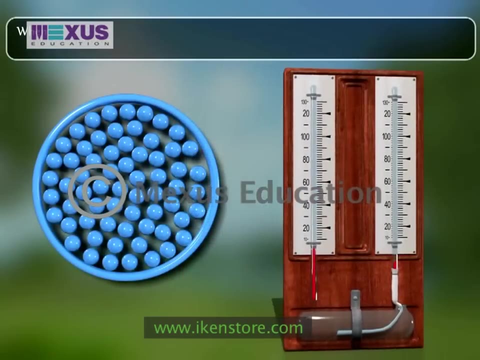 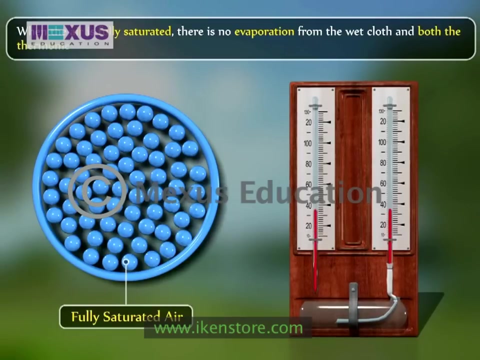 The difference between the dry and the wet bulb readings gives an indication of the humidity of air. The difference in temperature shown by the two thermometers increases as relative humidity decreases. When the air is fully saturated, there is no evaporation from the wet cloth and both the thermometers read the same. 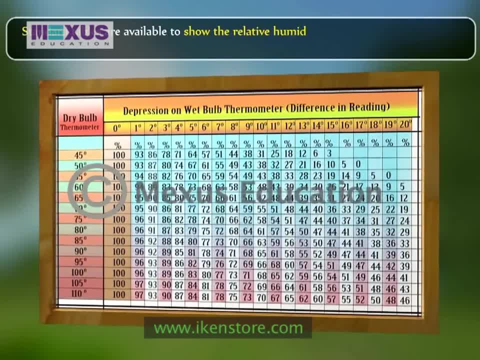 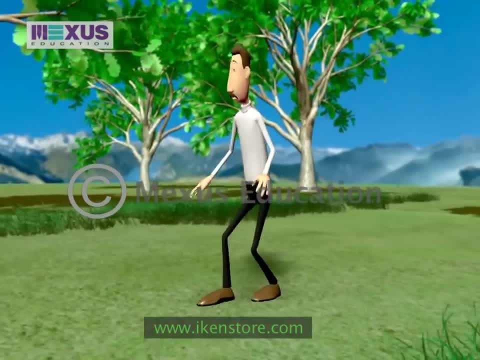 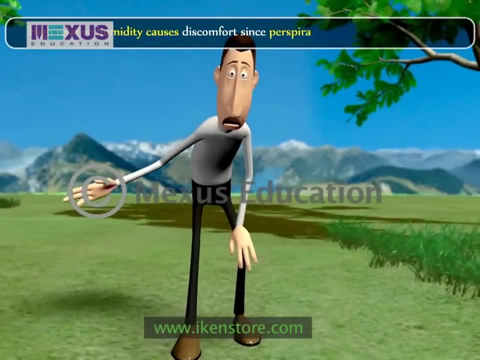 Standard tables are available to show the relative humidity for a given combination of wet and dry bulb thermometers. Humidity has a certain effect on our life. High relative humidity is a sign of high relative humidity. Humidity causes discomfort since perspiration does not dry up easily. 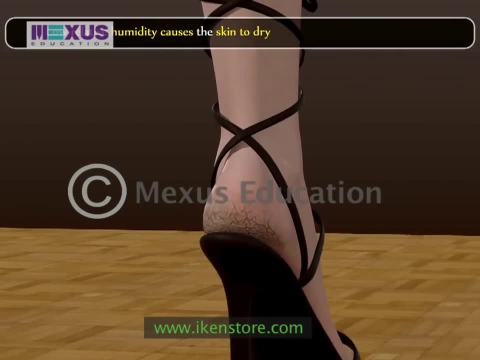 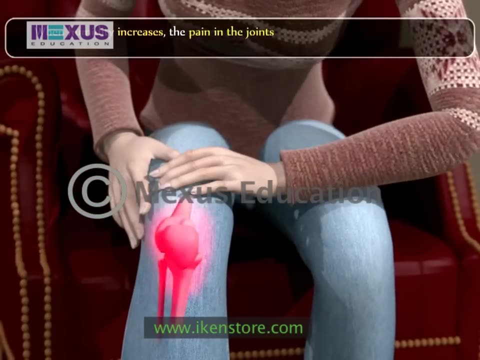 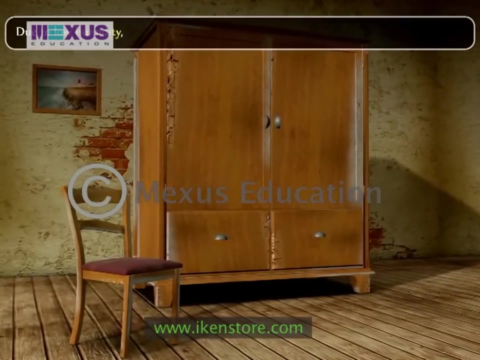 Low relative humidity causes the skin to dry and become rough and cracked. When humidity increases, the pain in the joints also increases. for people who are suffering from rheumatism Due to low humidity, wood and glue dries out, causing the furniture to loosen and crack. 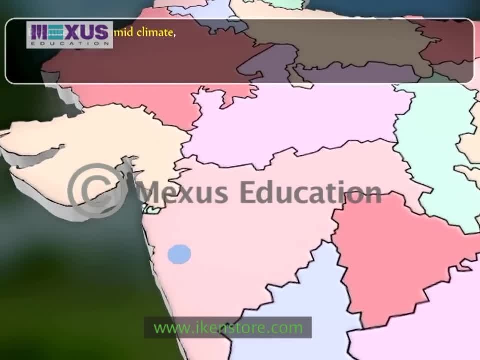 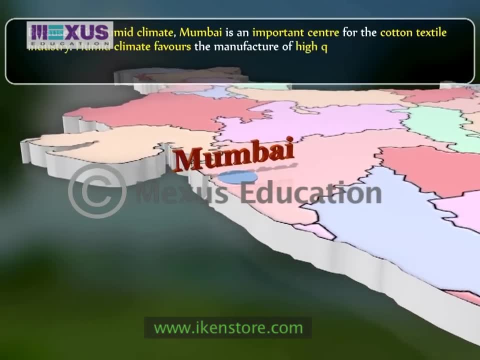 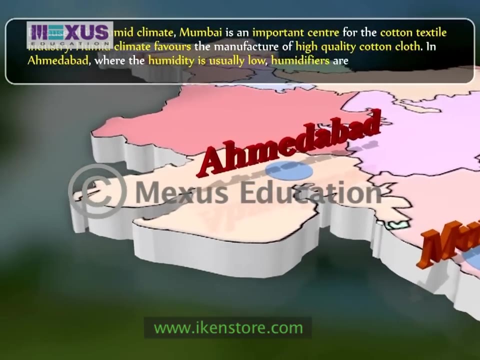 The temperature is also a sign of high relative humidity. Because of its humid climate, Mumbai is an important centre for the cotton textile industry. Humid climate favours the manufacture of high-quality cotton cloth. In Ahmedabad, where the humidity is usually low, humidifiers are used to regulate the humidity in its cotton textile mills.